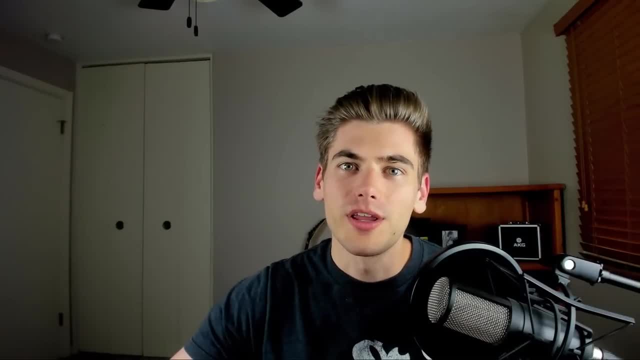 Hello everyone. In today's video, I'm going to be talking about regular expressions and I'm going to be going in-depth, covering everything you need to know about regular expressions. This includes the simple stuff, such as matchers, digits, selectors and so on. 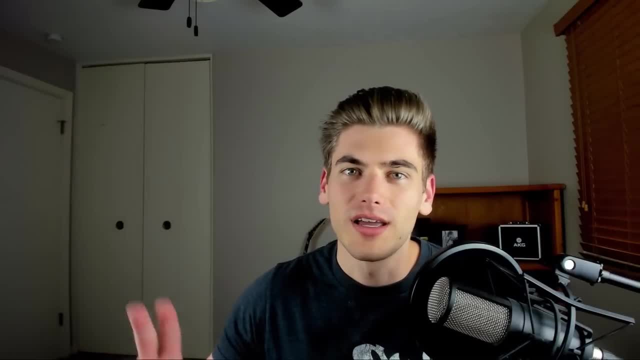 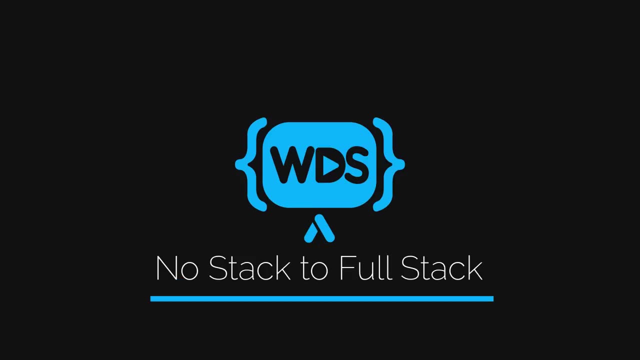 all the way up to more advanced features, such as capture groups, negative lookahead, positive lookahead and so on. So let's get started now. Welcome back to WebDev Simplified. My name's Kyle and my job is to simplify the web for you. 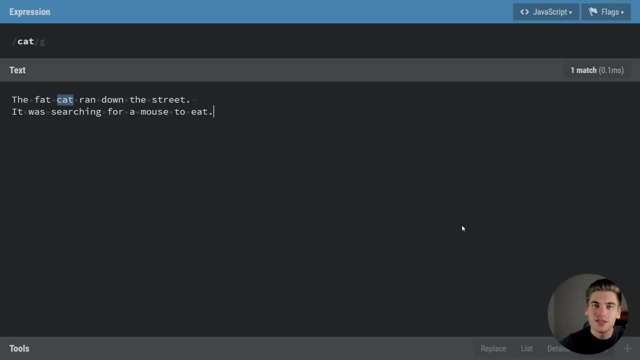 so you can start building your dream projects sooner. So if that sounds interesting, make sure you subscribe to the channel for more videos just like this one. And now to get started, I'm on a website here which really helps with regular expressions. I'm going to link it down in the description below so you can go to the same website. 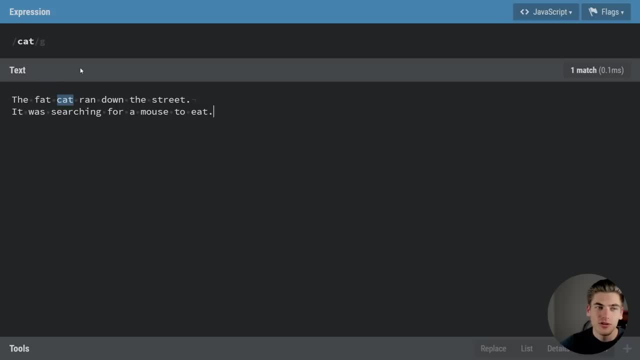 but it's really useful because it highlights, inside of the text you're searching for, what your regular expressions are. So I'm going to go to the same website and I'm going to go to the same website and I'm going to go to the same website. 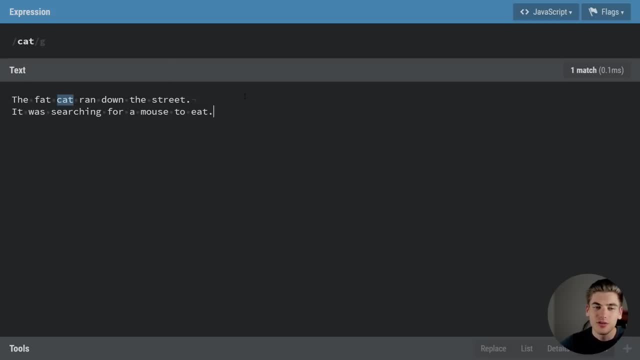 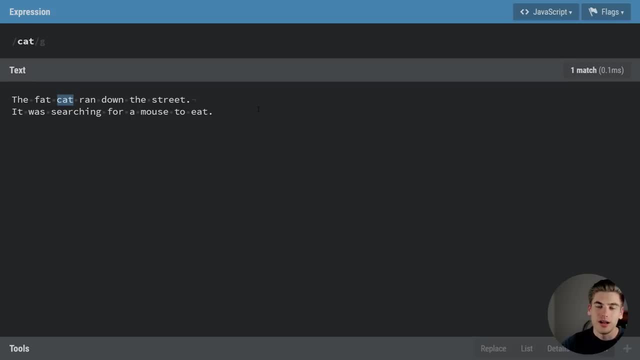 It's great for practicing and testing out regular expressions, so I highly recommend you go down to the link in the description and follow along on this site. And now to get started. I first want to explain what regular expressions are And essentially, a regular expression is a way to. 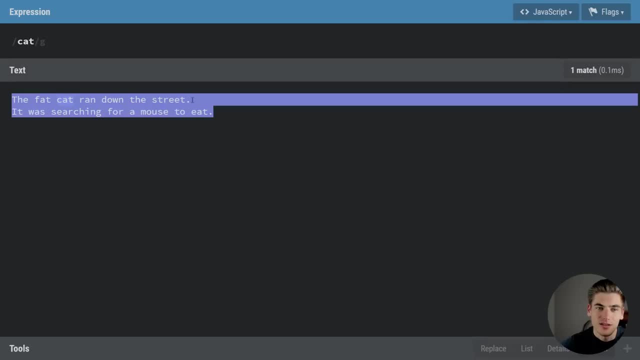 search through a string of text. So we have this text in here and at the top we have a regular expression, And what that regular expression allows us to do is it allows us to search through that text in order to do things such as validation or get certain pieces of the text. we can do advanced. 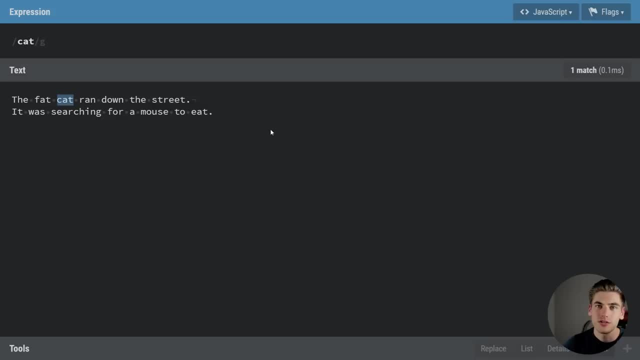 find and replace. there's a ton of things that you can do with regular expression, but in general, all that regular expression is doing is it allows you to search through text in a really advanced way and even group those different searches together so you can do powerful things such as find and. 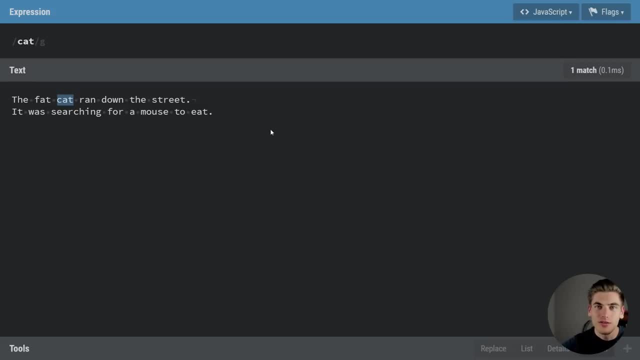 replace with it. so, to get started, i kind of want to break down the format of a regular expression. as you can see, up here we have our regular expression and in the middle here we have our text. we're searching and regular expression is almost always going to start with this opening. 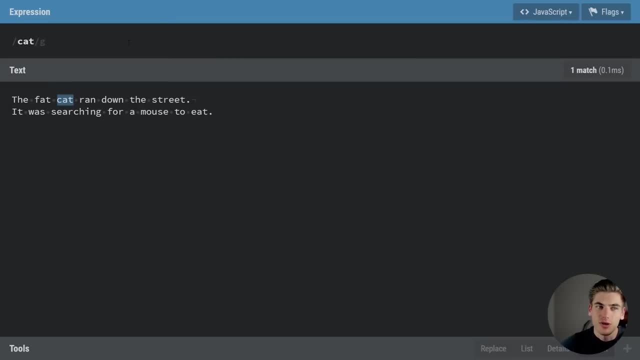 slash here, this forward slash and it's going to end with a forward slash as well. a lot of programming languages: when you define regular expressions, instead of defining them in sort of string quotations, you define them inside of these forward slashes. so everything between the forward slashes is going to be your regular expression, then also something that's a part of a regular 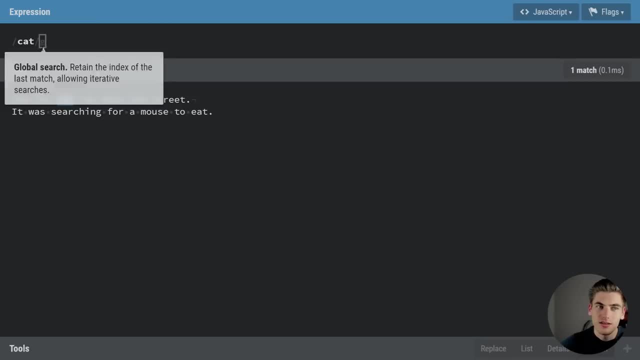 expression is the part after the forward slash here at the end. these are the different flags and, as you can see, we can access these flags up here and the main ones that you need to know about is global. this allows you to match anywhere in the string. for example, if we did at here, you can see that it matched all three of the different ads. 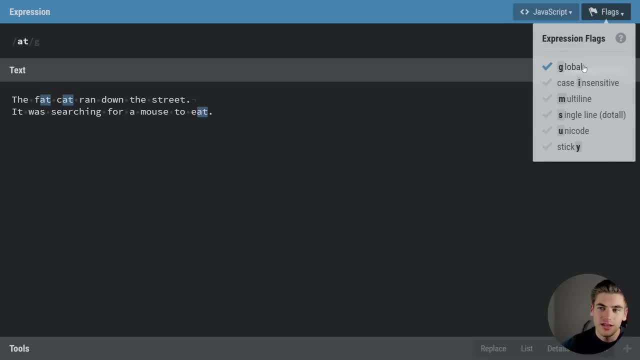 that's because we have global. it allows it to do multiple matches. but if we take global off, it's only going to match the first result that we find. so, essentially, global is like match all, while without global is like match one. next, we have case insensitive. so, for example, if i put 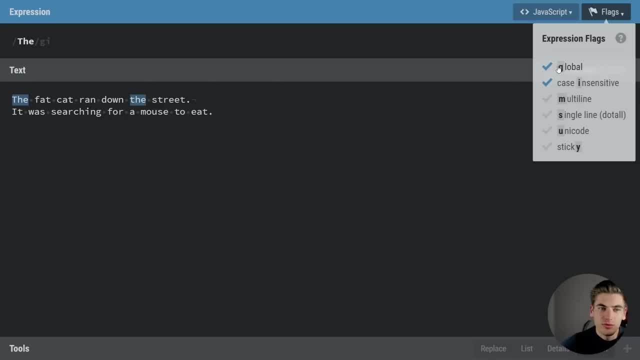 the with a capital th here, and then, if i make this global, you can see it's matching both of these. thus- and that's because i have case insensitive turned on- if i turn that off, it's only going to match the the that is capitalized, and if we change this to a lowercase, it's only going to match the lowercased one. 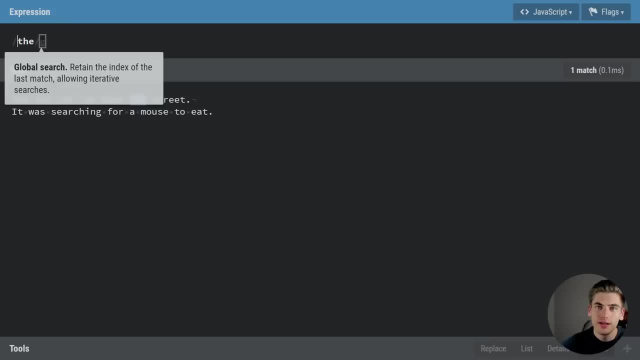 for the purposes of this tutorial, i'm just going to leave us on the global flag with case sensitivity, so that way capitals actually make a difference. and that's just because this is the most general configuration that you're going to use when messing with regular expressions and to get started. as you can see, this works very much like a normal find, if i 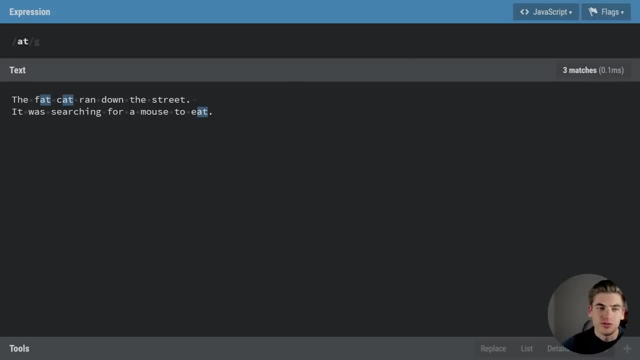 type information into here. whatever i type is going to be searched for in the string down here, for example, at i can search for fat and i'm just going to get the word fat, i can do ran and so on and it works just like normal find and replace, which is not really that powerful, but where it 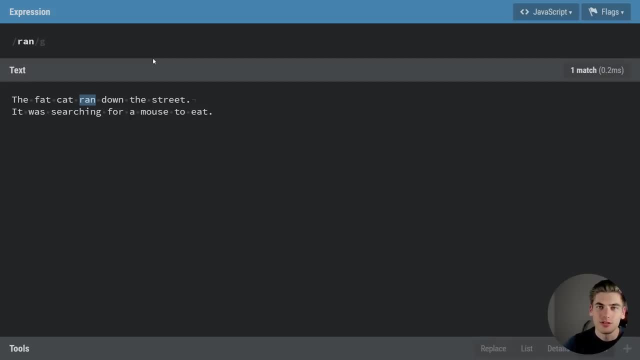 does become powerful is when you can actually start adding in the regular expression things, and the very first one that i want to talk about is the idea of these different special characters that allow you to do certain things. so, for example, we can search for the character e and you can see. 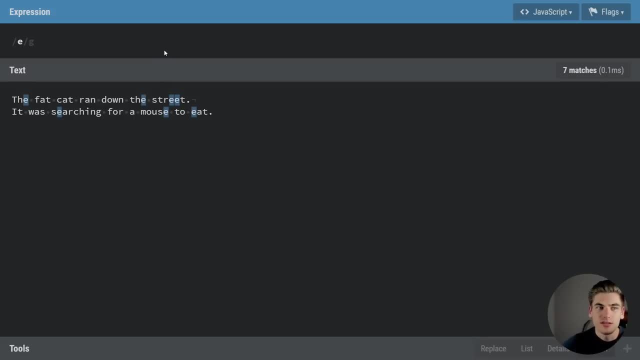 that we have a string of e's inside of our search. but what if we wanted to search for a string of e's, so multiple e's in a row, we could put e and then we could put a plus, and what this is saying is: it's saying match e, but we want to match at least one. this is one or more of the preceding. 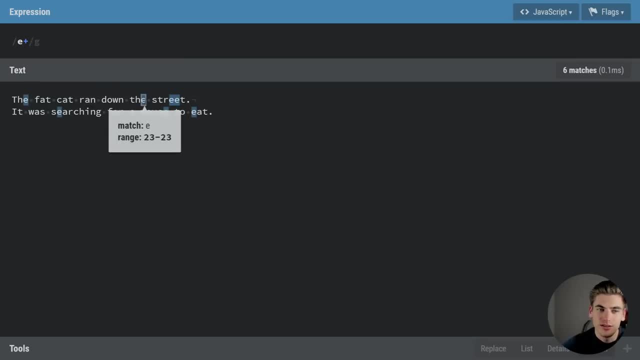 token. so we're saying match e or more than one e. so, as you can see, we have this e being matched this e, but this is actually matching both of our e's, because there's two e's in a row and the plus is just saying: match as many in a row as you can, but match at least one and then another character. 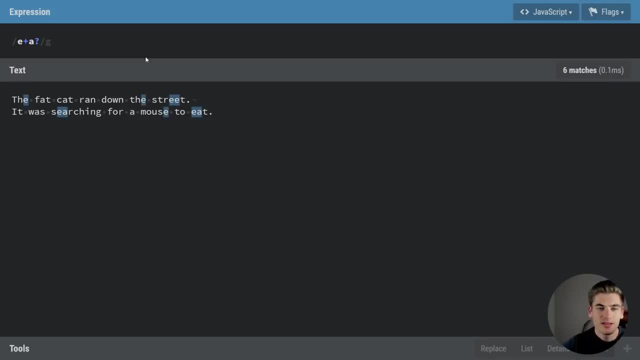 we can put an a in here and we can put a question mark, and that's saying that this is optional. so optionally i want to get this a character. so here we have ea, so it's going to get the character e, as you can see in all of these, and then if there's an a, it's also going to match that. 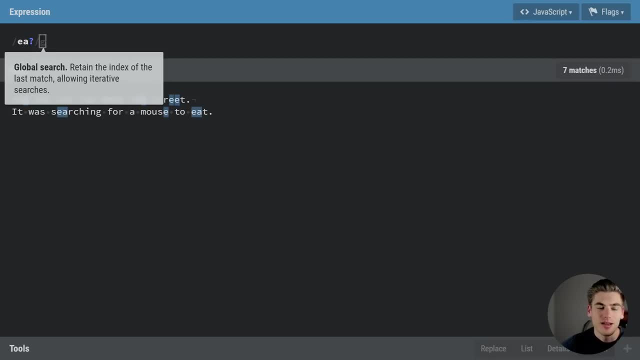 so this question mark says 0 or 1. i like to think of it as whatever is before it is optional. so in our case, our a is optional and wherever there is an a after an e, it's matching it, but in the case where there's no a after the e, it's just completely ignoring it. the next one that i want to talk. 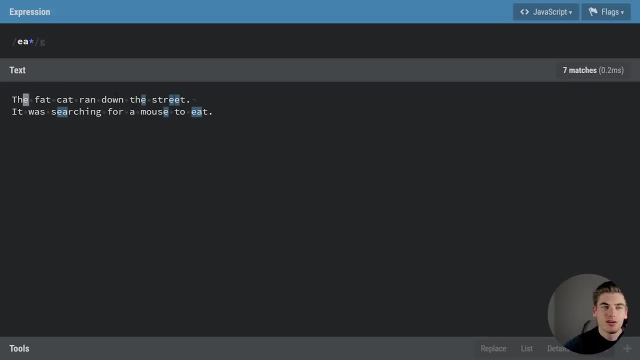 about is going to be here: the star indicator. and the star indicator essentially says: match zero or more. so it's kind of like a combination of the question mark and the plus. it's saying that it's optional, but you can match as many as possible in a row. so when we can see this is if we do r? e and 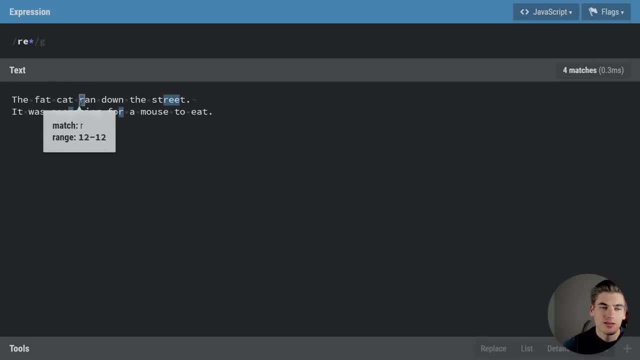 then, star, you can see it's matching anything in here that is an r, and then it matches all of the e's that follow it, if there are any, and if not, it just matches the r itself. another special character that's really important is the period character. 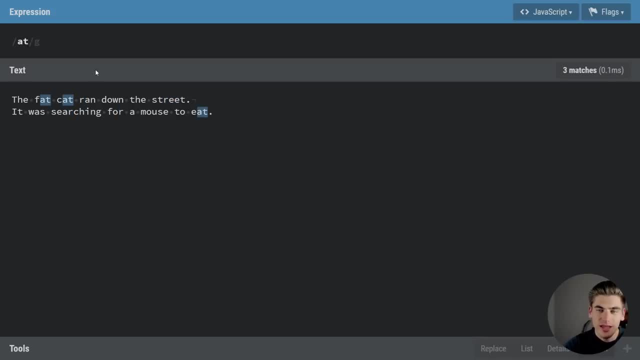 and the idea of the period character is that matches literally anything at all. so, as you can see here we put the period and it's matching the f, the c and the e. it doesn't matter, it'll match anything, except for a new line. it won't match a new line, so we have a new line right here. 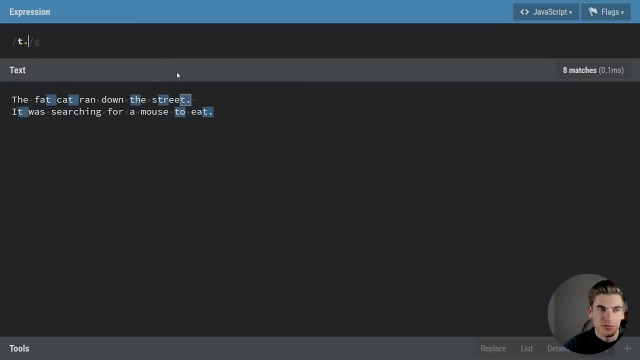 and if, for example, we wanted to search for t and then we want to search for period and we want to search for another period, you can see that it's not actually wrapping the new line, because period can't match a new line. also, you may notice that we want to search for a period, for example. how do we? 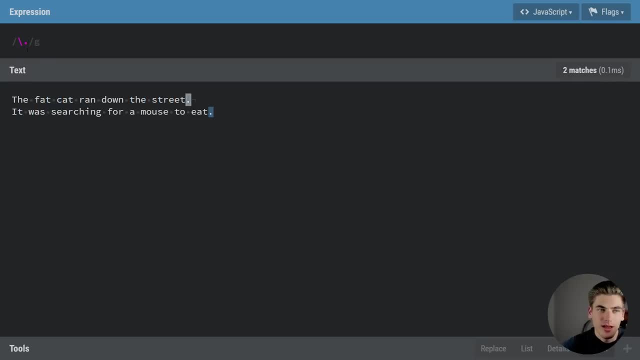 match all of the periods we can use here: the backslash and then the period. and what the backslash allows us to do is just cancel out anything that comes after it. it essentially escapes it. so, since we have the special character period after it, it's saying: treat this as a normal. 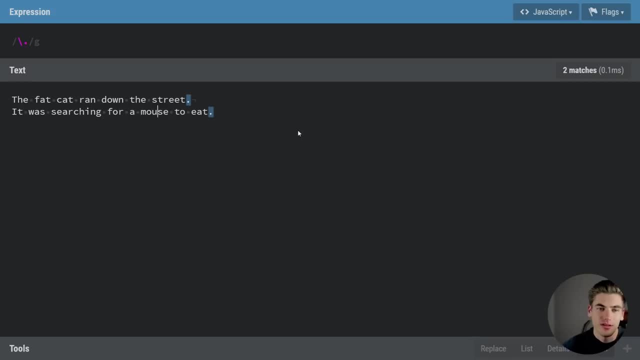 period and not as the special wild card period. that matches everything and, as you can see, we're able to match any of our periods and if we wanted to say let's match any character that comes before it, we could just put a period and now we're matching any character that comes before a period. 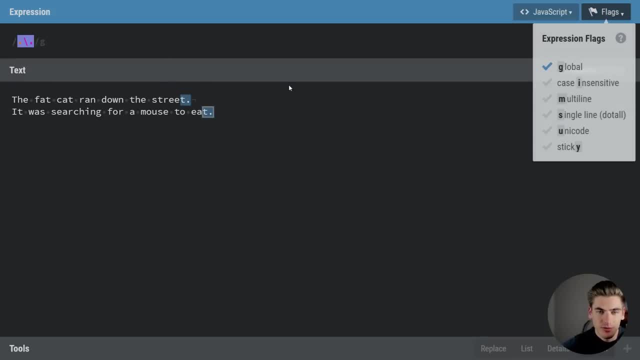 as well as the period. another really important special character that we can actually match any word character is going to be the slash w, and this is saying match any word character. so this is going to be things like letters. as you can see here it's matching every single letter in our list. 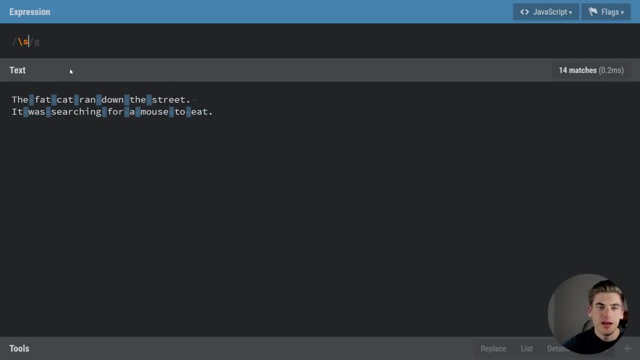 also there's the slash s. this is going to match any form of white space that there is, and the nice thing is these have negative versions. so capital s is going to match anything that's not a white space. capital w matches anything that's not a character, such as these letters here: 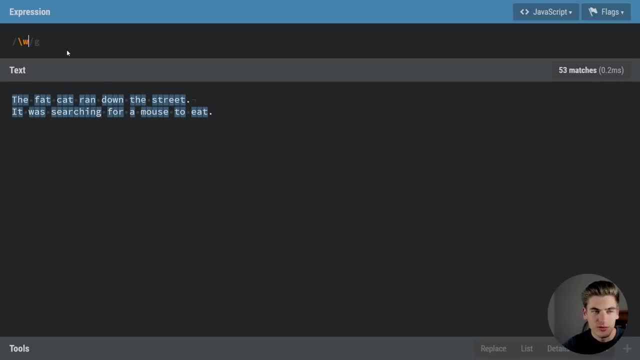 and let's say we wanted to capture all of our periods and we wanted to match all of our periods. so here's what we can do in the stardew forest strategy is to pick up a bunch of characters which will be the same number as the first four, and then say multiple characters that you'll 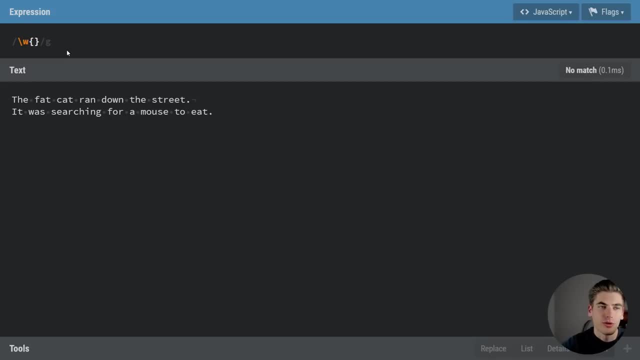 check out and do a search, and then you can use stardew forest strategy to actually keep track of all the words that are longer than four characters long. well, we can't use the plus, we can't use the star, these don't actually work. but what we can do is inside of curly braces we can. 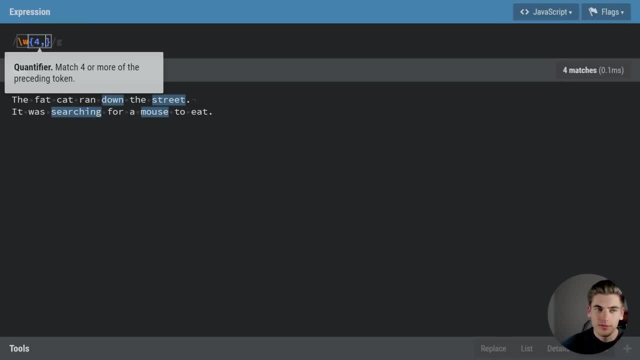 put a minimum and a maximum number for how large we want something. so, for example, let's say we wanted to get all the words that are over four characters. we could say four, and this is going to get us any four digits in a row, and if we put a comma it's going to say get any four digits or more. 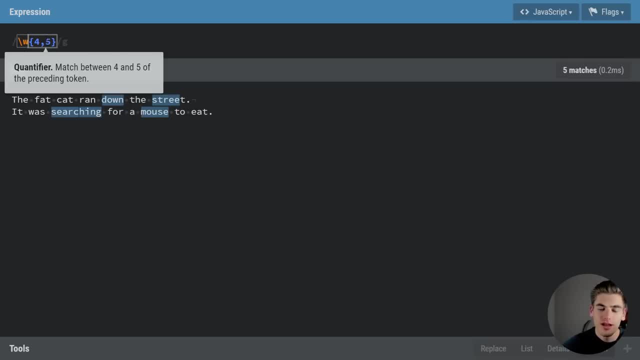 five, and it's going to match any set of characters that are between four and five long. And that, right, there is pretty much the majority of all of your counting selectors, as well as your special character selectors that you have to worry about. But another thing that you can do is actually do. 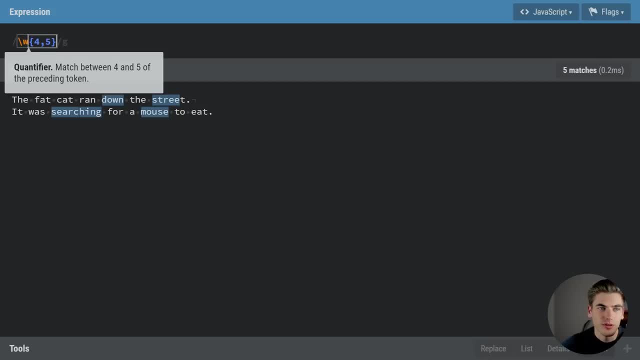 character groupings So we can get all of the characters inside of a group. So, for example, let's say that we wanted to get any single word that ends in AT and we wanted to get a three letter word that ends in AT, and we wanted to get only the words that start with either F or C. 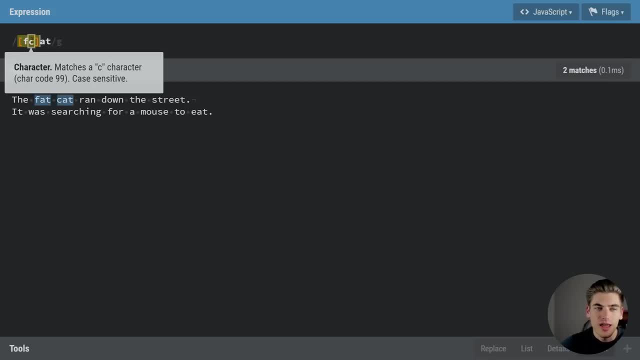 What we could do here is, inside of square brackets, we put any characters that we want to match And it's saying: match any of the characters inside of here. For example, it's going to match anything that starts with F or a, C and ends with an AT. But the really useful thing about these- 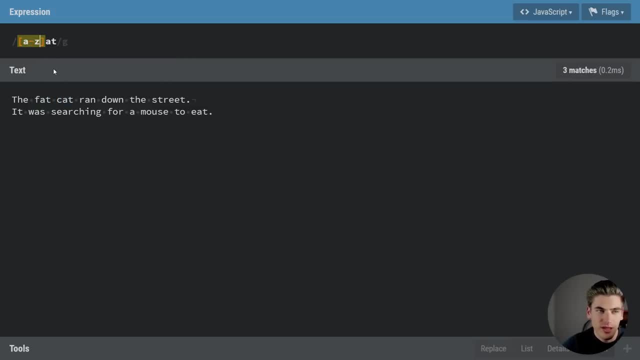 character sets is you can actually do ranges. So we could, for example, do A to Z, And this is going to be all of the characters between A and Z. We could also do between capital A and capital Z, And now we have all of the characters between A and Z that are lowercase, and all the characters. 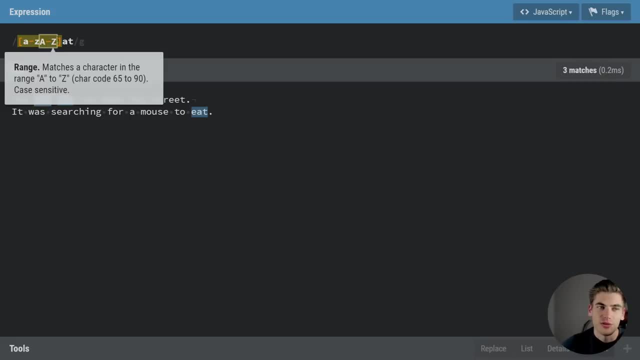 between A and Z that are lowercase, And now we have all of the characters between A and Z that are uppercase, that are going to be checked inside this regular expression. We could do the same thing, for example, with zero to nine, if we wanted to. It's really useful because we can do these. 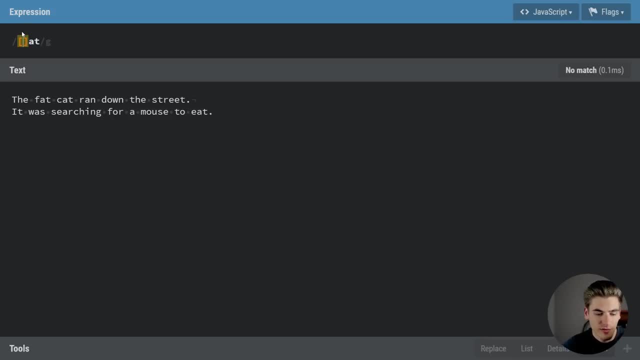 large ranges which allow us to do these really specific checks. For example, we could do like A to F and it's going to get anything between A and F. Or we could do A to C and we're just going to get cat now. in that case, Something else that's really useful is the ability to put things inside. 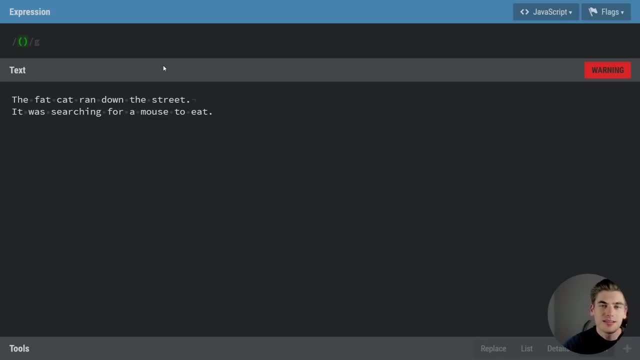 of a group, And that's what we use parentheses for. Anything inside of the parentheses are going to be their own group and they only act upon themselves. So, for example, we could search for T or uppercase T- Whoops, uppercase T And. 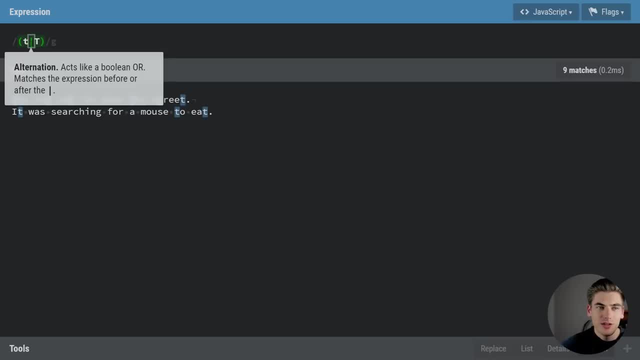 what this does, this little pipe character here- is it's saying: match any of these. So it's like an or result. It's saying either lowercase T or uppercase T, And then we want to match H E afterwards. So this allows us to match uppercase T or lowercase T and it's going to allow us to. 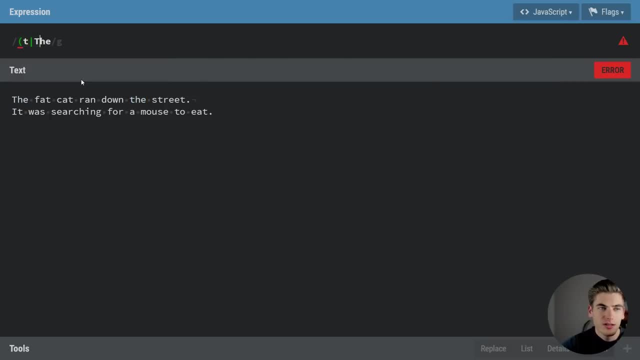 match it for the word the. And the reason we need parentheses is because, if we remove these parentheses, this character here is going to check for either lowercase T or uppercase T, Because it's going upon the thing on the left and the thing on the right, But with the parentheses. 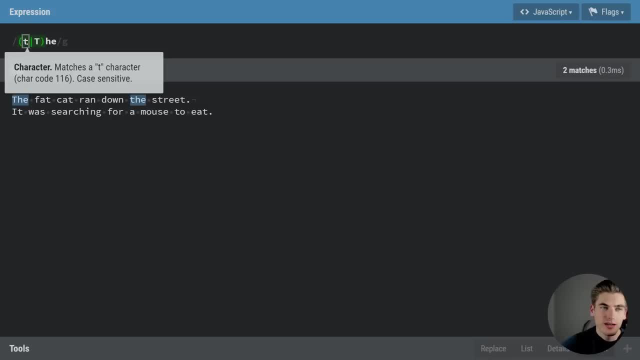 we can actually break this up into its own group. So now it's only acting upon the T and the uppercase T instead of the full word, the. Also, something that's really useful with these groups is we can actually do some things, such as our matches, where we could say we want to match for 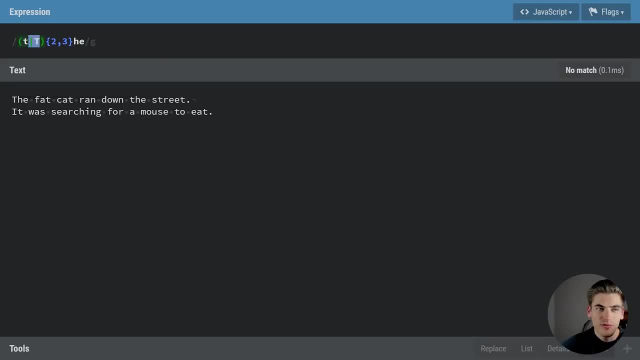 example, two to three, And it's going to say we want to match two to three of this character grouping here. So either lowercase T or uppercase T. So we can actually see this in effect, by doing if we want T, E and R, you can see it's going to. 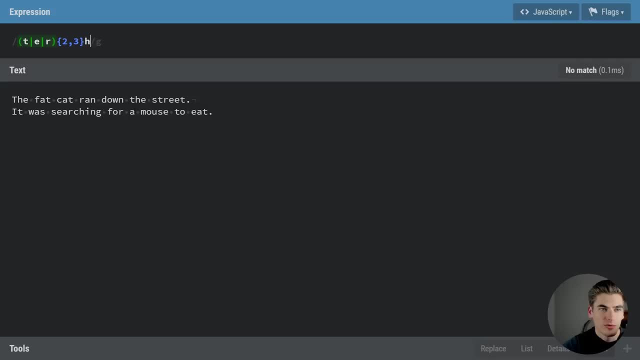 match between two and three of these. Let's just say we want to match between two and three of those, And you can see it's matching over here: T R, E, because it's in this group There's at least three of these, And then E T because there's two of them. And then, for example, we could even put: 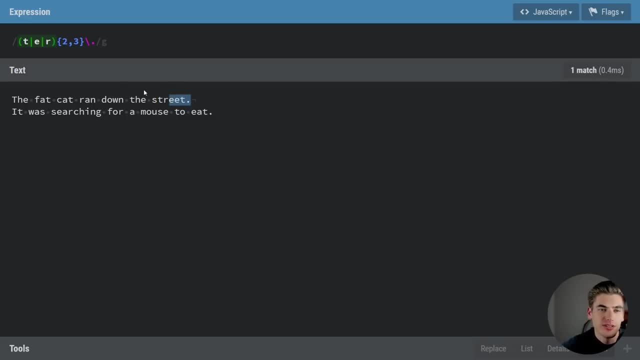 things after this. For example, we want to match the period key And you can see it's giving us the E E, T period at the end because it's checking between two and three of these characters up here in the beginning And then it's saying the actual. 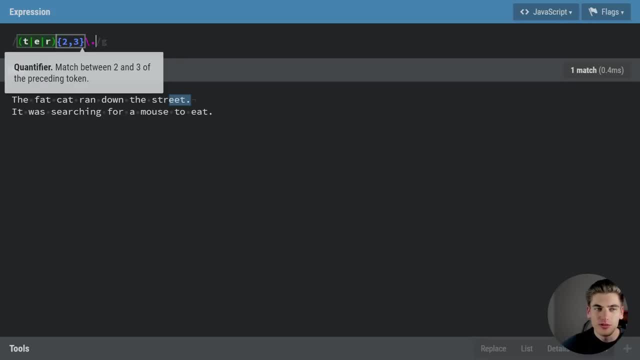 period key is coming after it. So with these capture groupings, what we can do is we can actually specifically say we want to do special things only to those groupings. So anything that we put after these groupings are going to affect the entire grouping and not just a single character. 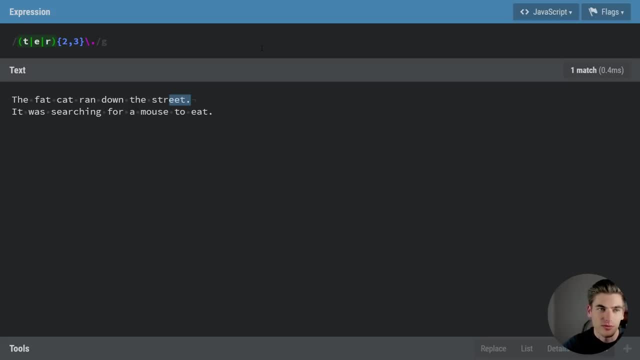 inside of that grouping, as we were doing before. Because, for example, if we remove all of this, we just change this to, for example, E of two to three, What this is doing is only acting upon this E, And if we put, for example, an R in here, it's not acting upon this R at all. This R is 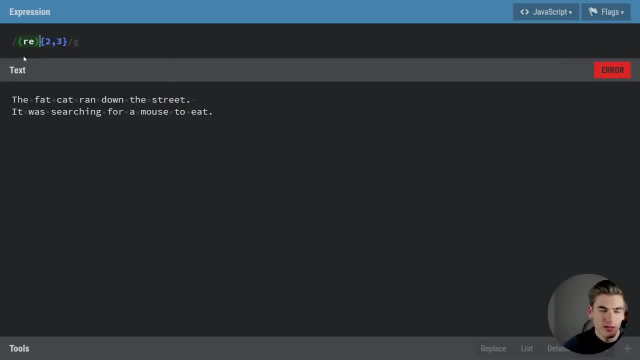 completely separate from this E, And if we put, for example, an R in here, it's not acting upon the E. But if we were to put it inside of a group like this, now, what this is saying is any set of RE. 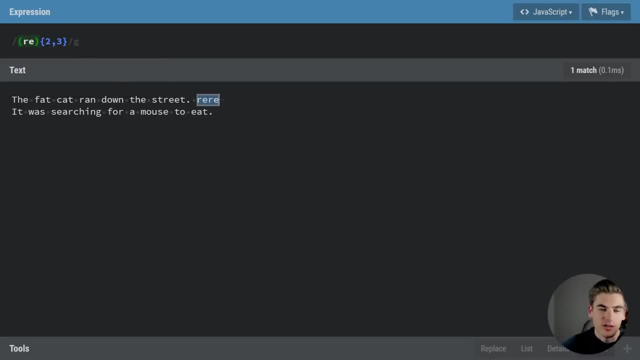 that is seen in a row two to three times. So, for example, if we put R E R E, you can see that's going to match it. We put another one, it'll match it, But of course the fourth one will not. Now, 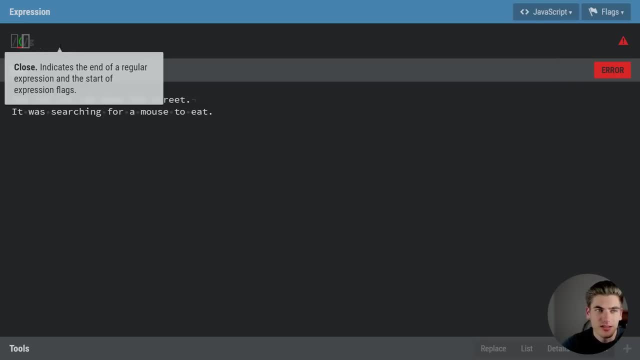 another special character which is really important to get used to is the caret symbol, which essentially says match the beginning of the line. So, for example, we put the T here, It's going to match the beginning of our statement, But if we put a capital, I and the caret symbol. 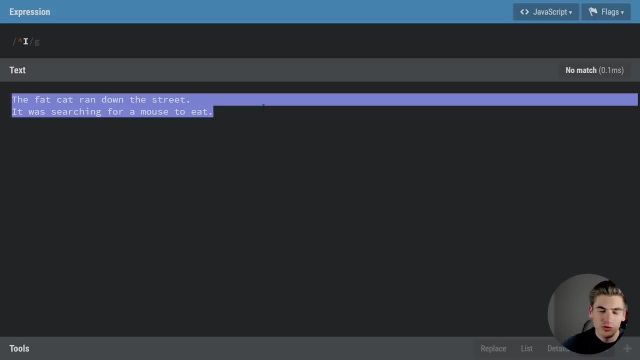 it's not working And that's because we are doing this as one whole chunk of text, So this caret is the very beginning of our entire chunk. If we wanted to do it per each individual line, we would need to set the multi-line flag, And now that's saying that this caret symbol is. 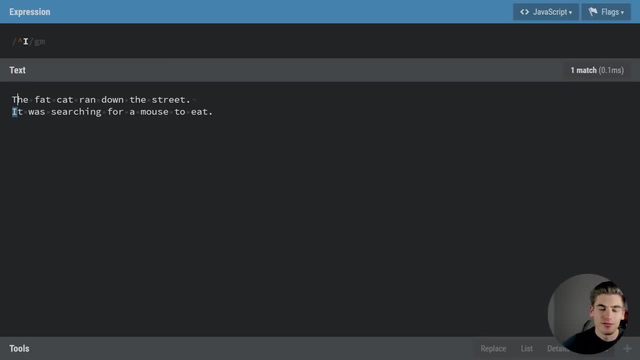 the beginning of each and every line that we have, instead of just the beginning of the actual statement as a whole. I'm going to turn that back off just so that we know that this is going to be the very beginning of our entire statement. So, for example, our T is going to match this T here. 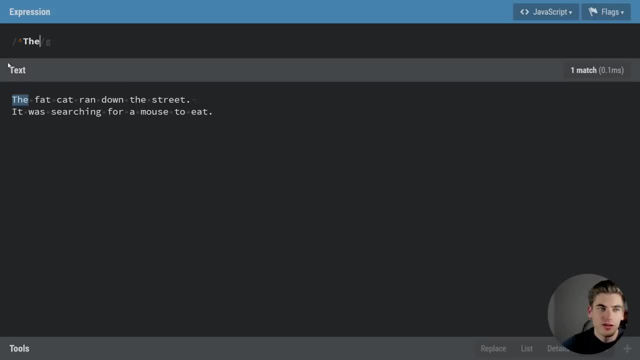 And we could put, you know, for example, a button. It's going to match that whole word, the, but only going to match the the at the very beginning, even if we made it so that it could be a lowercase T by doing this. So it could be either. 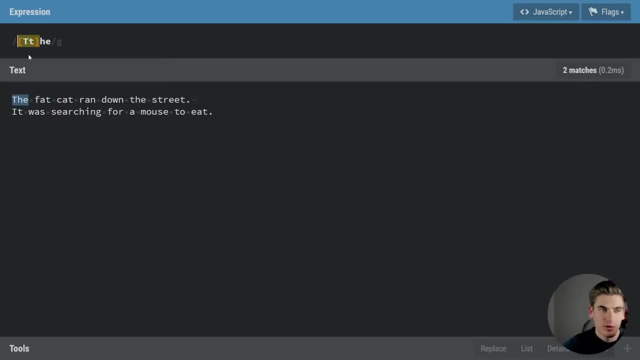 an uppercase T or a lowercase T, You can see it's still not matching. But if we remove this, you can see now it matches both of those. Another thing that you can do is the dollar sign symbol, And what this is saying is match the end of our statement. So, for example, at the end we have 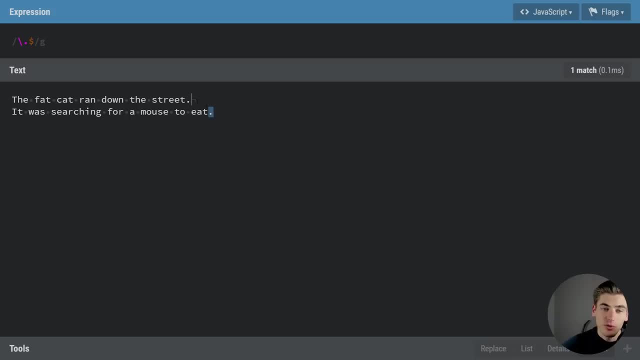 a period And you can see it's matching this period here, But of course it's not matching the period at the end of street because we would need to enable multi-line. So that way this works on the end of the line instead of the end of our entire statement. But 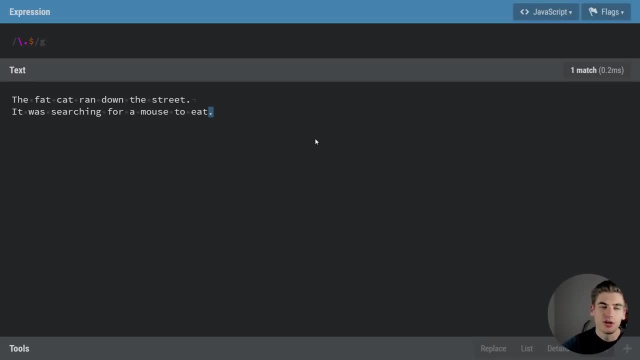 again. I'm going to turn that off just because I think it's easier to work with when you use a whole statement instead of multi-line, at least for our examples. Now, that is essentially 90% of all of the regular expression stuff that you're ever going to use. You're really only going to 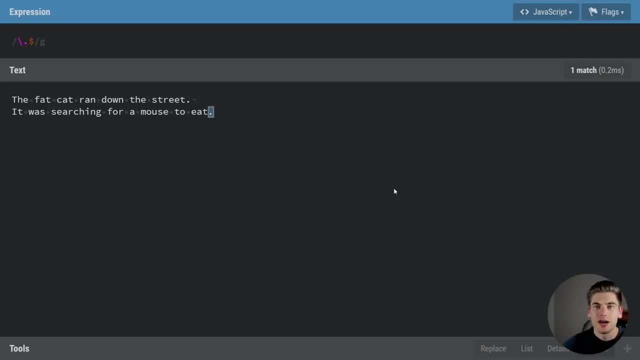 use these genericish matchers as well as capture groups in order to make these complex selectors, But something that you can use that really increases the ability of you using regular expressions is look aheads and look behinds, And to get started, I'm going to talk about a look behind. 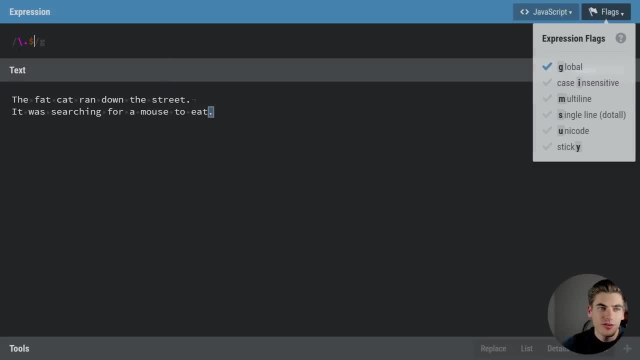 first- And we're going to talk about the positive look behind And the way that you use a positive look behind is you need to put it inside of a group, And this group is going to start with a question mark, as well as the less than sign and then the equal. So this is saying that we want to 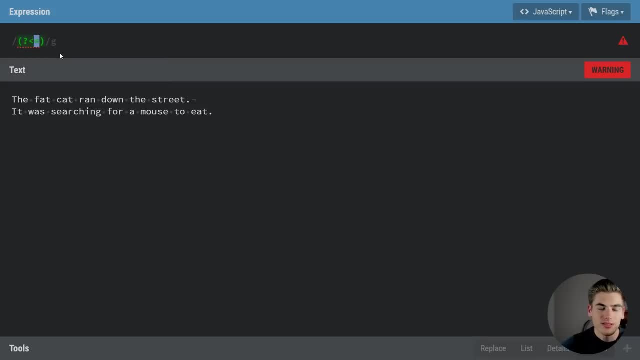 look behind us. That's what this less than sign is. And then the equal is saying it's positive, So it must match what's inside of here. So, for example, what if we want to get every single word that is followed by the word the? 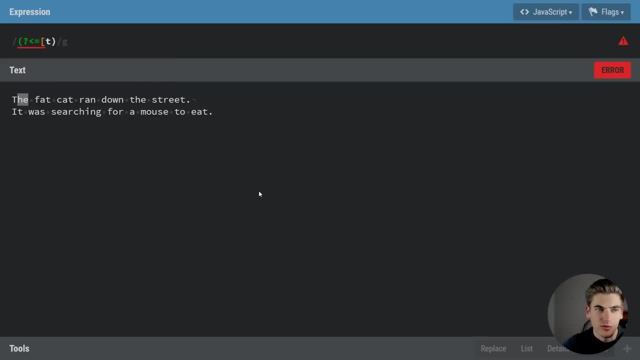 We can come in here and we can say that we want to match either a T or an uppercase T, and we want to match H, E, And we can just say: we want the very first character that's followed by the word the. So we'll. 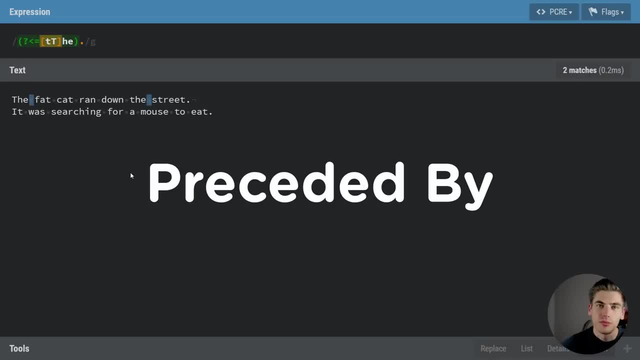 just put a period here And you can see we're getting both of the spaces that are followed by the, But we're not actually getting the word the inside of our selection. As you can see, it's only the period, And that's the value of these look aheads and look behinds. is they allow? 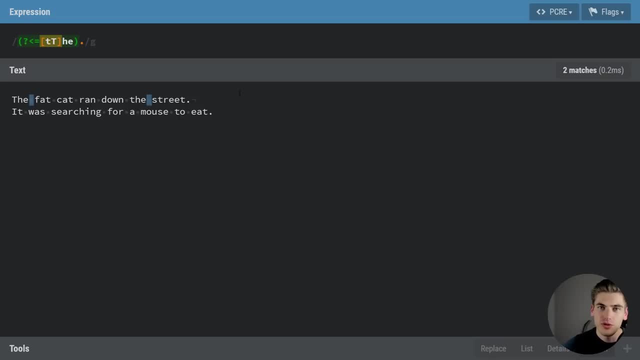 you to look at things that either happened before or after the thing you want to capture, But it doesn't actually capture or select the thing that you're looking behind or looking ahead for, And that's super useful And I really like that about these, So we can say that we want. 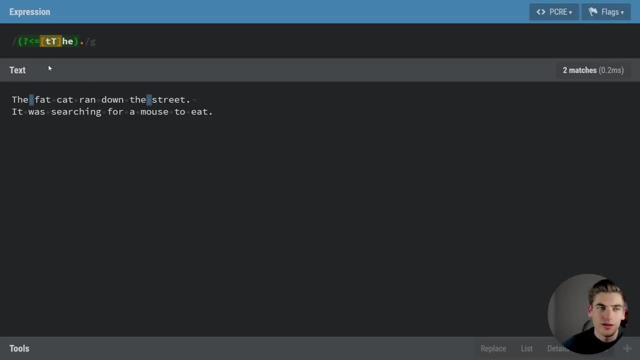 something followed by the word the, But we don't need to select the word the. Also, there's the negative look behind, And this is going to be. replacing this equals with an exclamation point, And this is saying that we want to get anything that doesn't have the word the before it. So 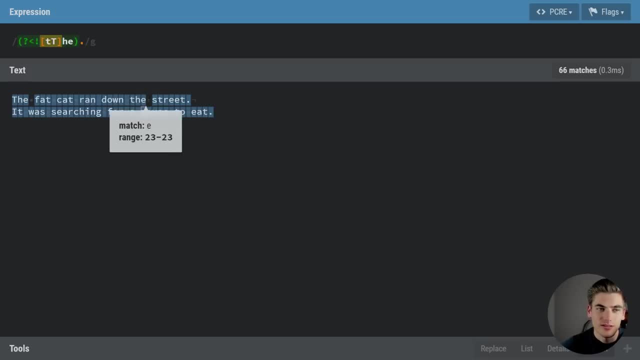 you can see it matches every single character, except for the two spaces that had the word the before it. The negative look behind is pretty much identical to the look behind. that's positive, except for it's just going to invert it. So your results are going to be completely inverted from. 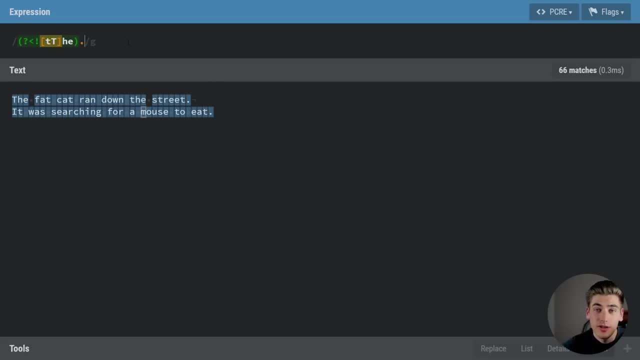 the results of the positive look behind. Now we can move on to the look ahead, And look ahead is very similar to look behind, but we just remove the less than symbol. So let's come in here and we can do a look ahead. that's positive first, And we want to say that we want to get anything that 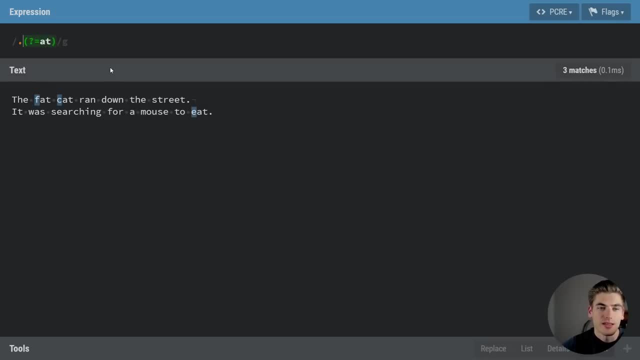 has an at after it. So we want to get any character that's followed by at And. as you can see, we've got a function, So we want to change that to a And we want to convert that to a. 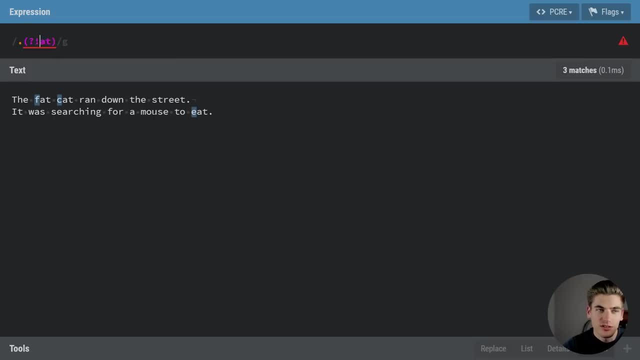 And if we want to invert that, we just change. this equals to an exclamation point And, as you can see, we're now getting everything that's not followed by at, So everything but the f, c and e. Now that we understand all of the basics of regular expressions, let's actually look into 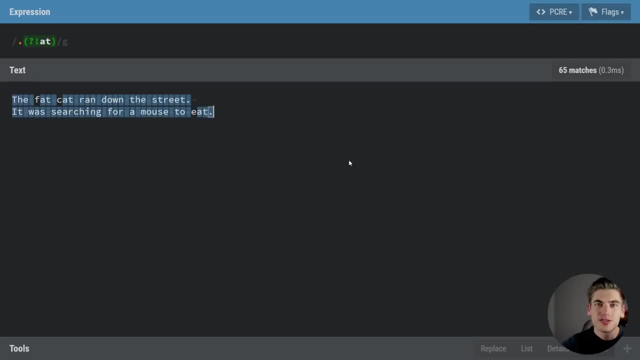 implementing a regular expression to check for a phone number. This is a great example because it can be really simple, But as you start to add different types of formatting to your phone number, it can get really complex and allow you to build on your regular expressions. So let's go. 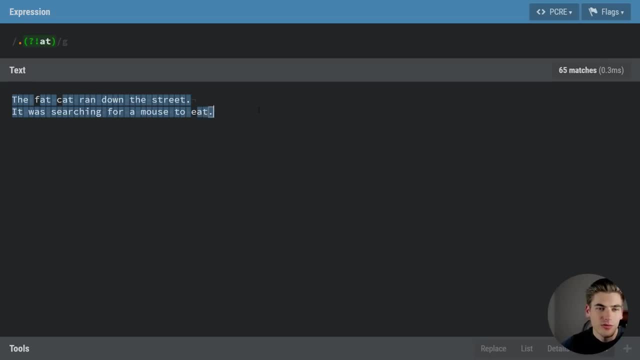 right ahead and get this big base. So let's go ahead and get the code here And let's say: we've got a skills as you go, So let's come in here. replace all this with just a random phone number. We'll. 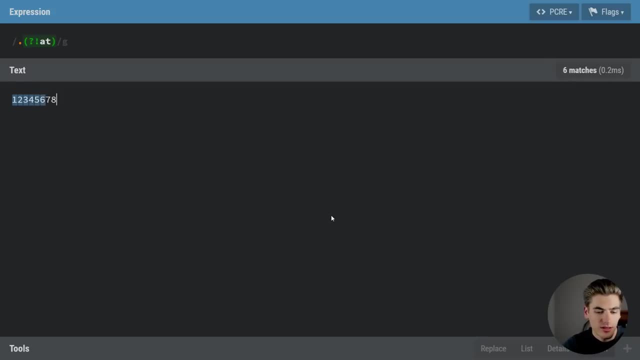 just say 1,, 2,, 3,, 4,, 5,, 6,, 7,, 8,, 9,, 0.. So we have our area code of three digits and three more digits and then our last four digits. This is going to be the easiest phone number to check for, because 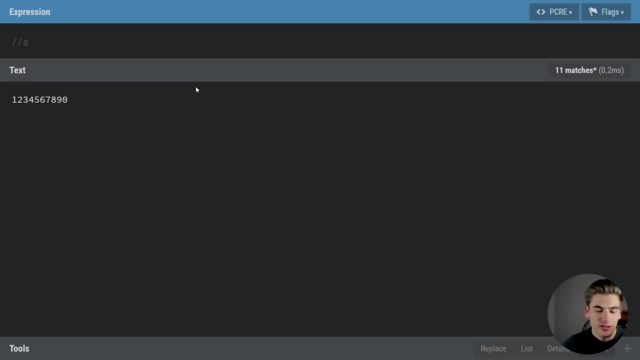 all we need to do is just check for nine characters in a row, So we can just say slash D, which is going to be for digits. This is any form of number digit And we can just say that we want to get nine of them in a row. I'm sorry, we need to make sure we get 10 of them in a row, because 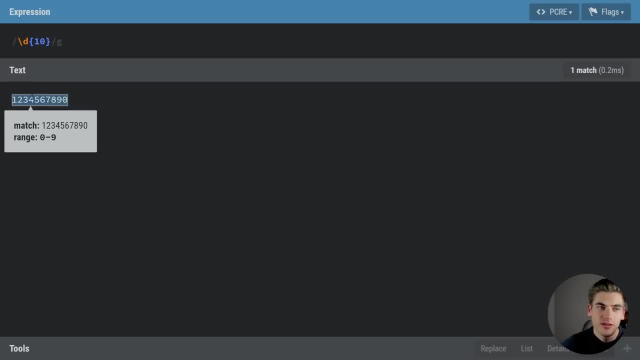 this is a 10 digit number And, as you can see, that's matching that perfectly, But obviously there's multiple different types of phone numbers that we can search for. For example, we could have the phone number 1, 2,, 3,, 4,, 5,, 6,, 7,, 8,, 9,, 0. And we also need to be able to account for that. 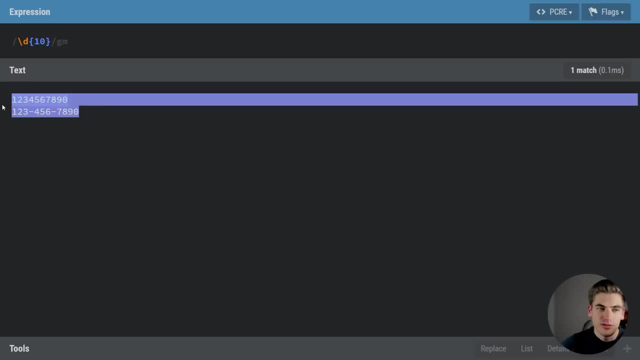 And now I'm going to enable multi-line here, because now we can actually search each one of these lines individually to make sure that they all still work. So now, instead of just being able to check for 10, 20 characters in a row, we need to check for groupings. So the first thing we're going to have 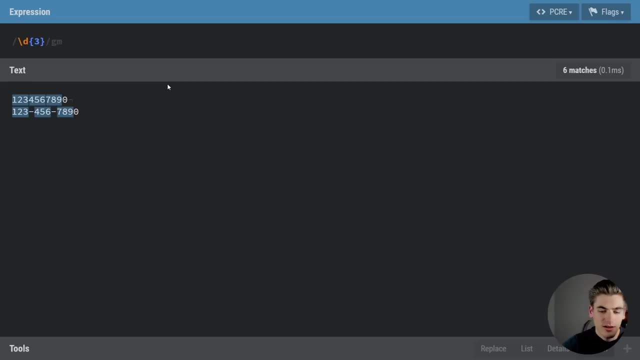 is a set of three characters in a row for our digit, And then we're going to have a dash. but we want to make sure that dash is optional, So we put the question mark. Next, we're going to have another three digits in a row, So we're just going to come in here, say the D, and we're going. 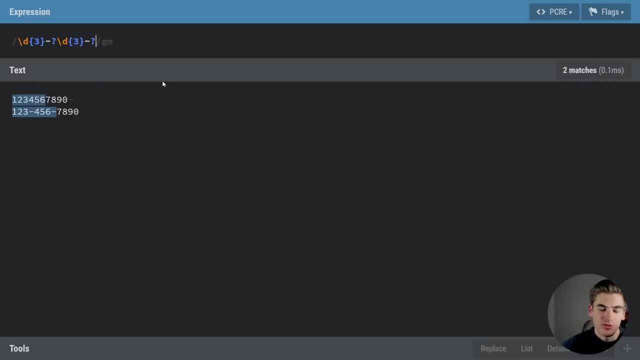 to have three more in a row And again an optional dash. So we'll put dash with the question mark to say that it's optional. And then, lastly, we're going to do the same thing. We're going to have our digits and we want to have four of them this time instead of three. 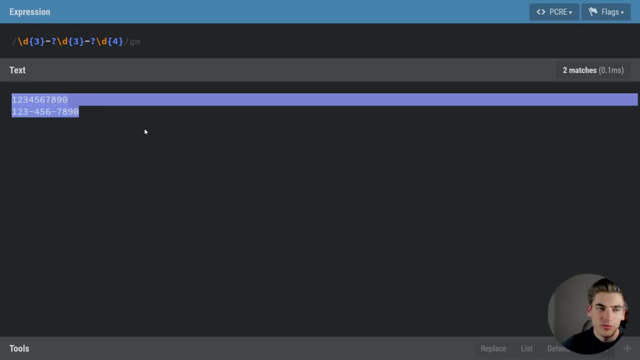 And there you go. We now have matched both of these different types of phone numbers. Now, obviously, another way for someone to write this phone number would be 123, space 456, space 7890.. This is also common, So we again need to account for that. We can come in here and 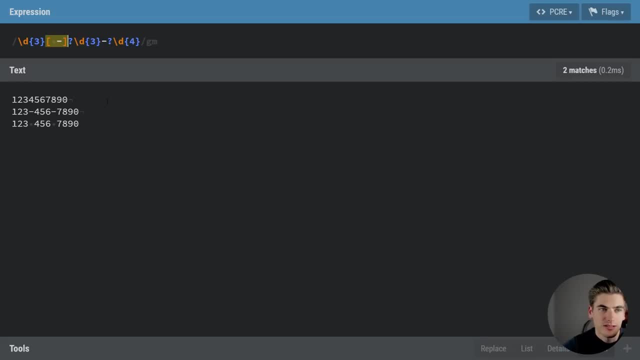 essentially put this inside of a character grouping and we can just put our space inside of it. So now we're saying any form of space between these, we can just do the same thing here We want to use space or dash, And now you can see we've matched both of these, which is great. 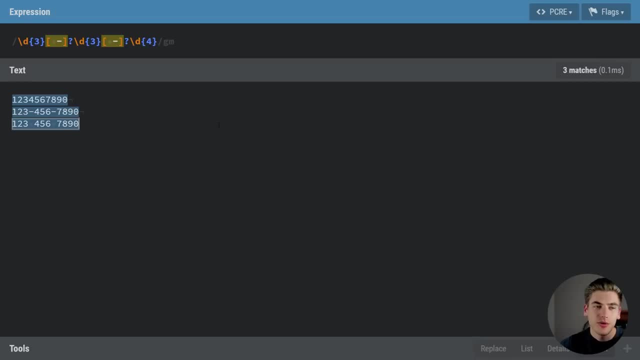 Before we get too carried away, let's say that the end result is that we want to take any phone number that we're given and convert it to just 10 numbers in a row, with no spaces, no dashes, no parentheses. What we're going to need to do is we need to capture all of our digits So we can. 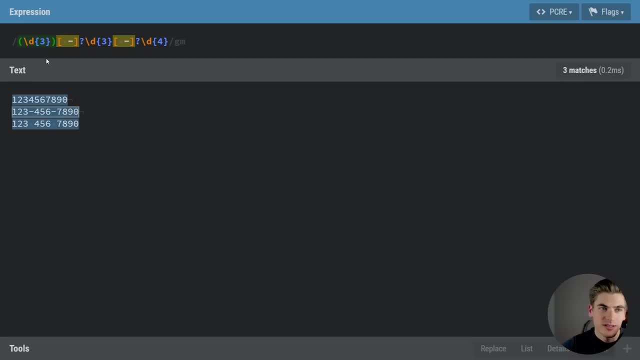 again, use capture groups for that. If you remember, when we put things inside of parentheses it's actually going to capture those, So we can put all of our digit segments inside of parentheses here And now. if we come down over into the details section, you can see that it shows all of our different 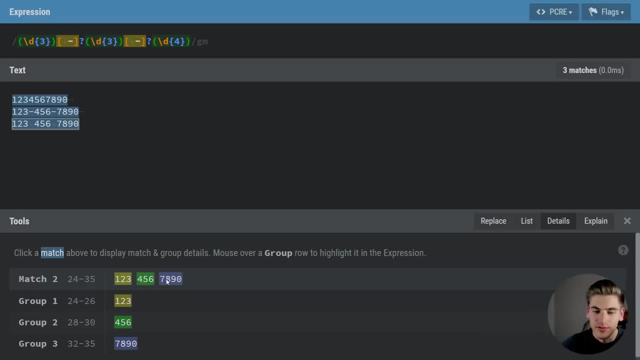 matches And you can see that we have matches of 1,, 2,, 3,, 4,, 5,, 6,, 7,, 8,, 9, as well as the different groups, And if we select here, you can see it's the exact same thing. It's matching 1,, 2,, 3,, 4,. 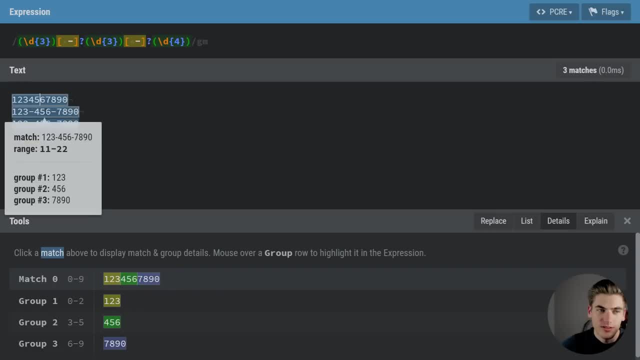 5,, 6,, 7,, 8,, 9,, 0.. And again same thing right here. When we click on these different results, it's showing what it's matching for each one of those, So we know that we're matching those. 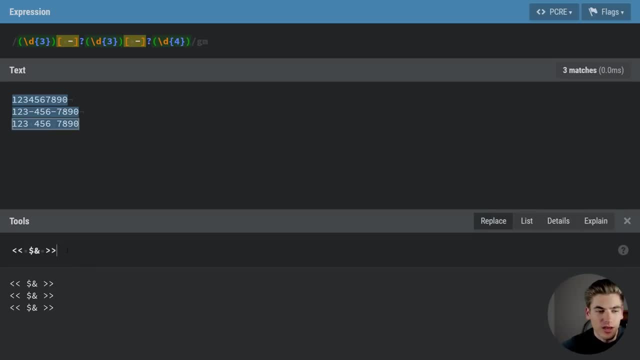 correct groups And we can come into replace, for example. And what we can do is we can say that we want to take group number one, So $1,, $2, and $3.. That's saying, take group one, group two. 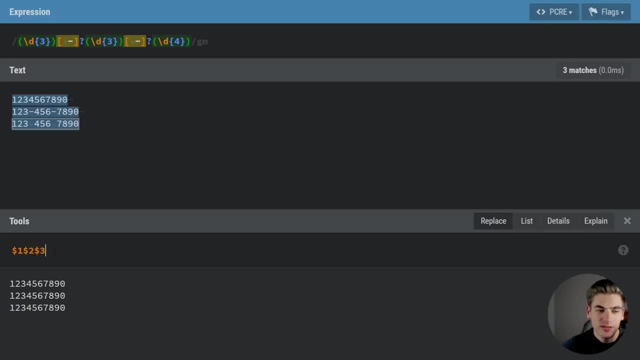 and group three and just put them one after another. And this is what happens when you don't name your groups. But you can actually name your groups by putting a question mark as well as the less than and the greater than symbol, And then inside of here you put your name. So, for example, 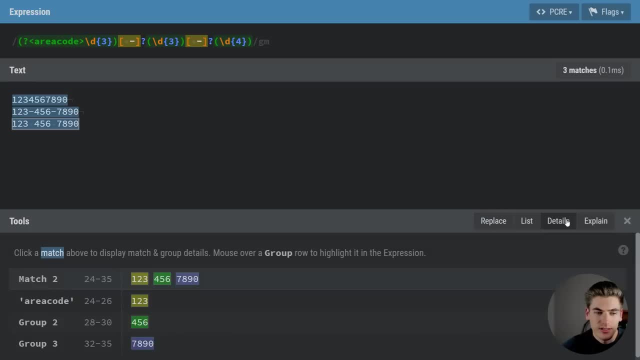 we can call this area code. Then we can come and look inside of our details section And you can see our area code is set to 1,, 2,, 3.. We can also name these other groups if we really wanted to. 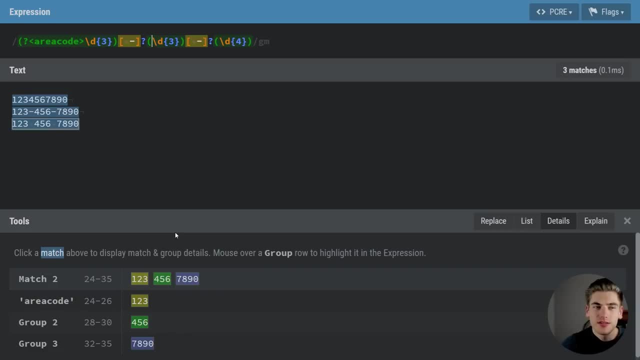 But it doesn't really matter. Naming them is more for convenience of use when you're actually going for find and replace and doing other complex things like that. Now let's go on and look at another example where we have 1,, 2,, 3.. And then it's going to be followed by 4,, 5, 6,. 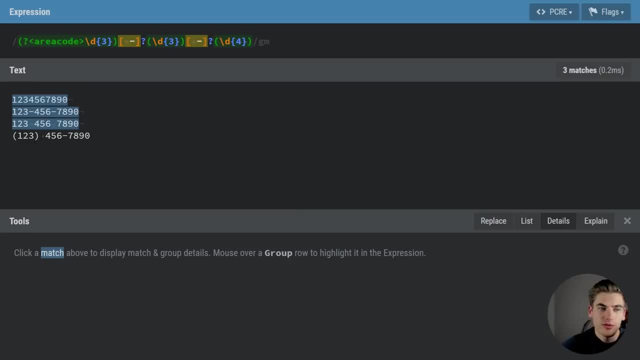 and then a hyphen and 7,, 8,, 9,, 0.. So now we need to account for parentheses around the area code, which again are going to be optional, So we can come in here, put a parentheses And we need to. 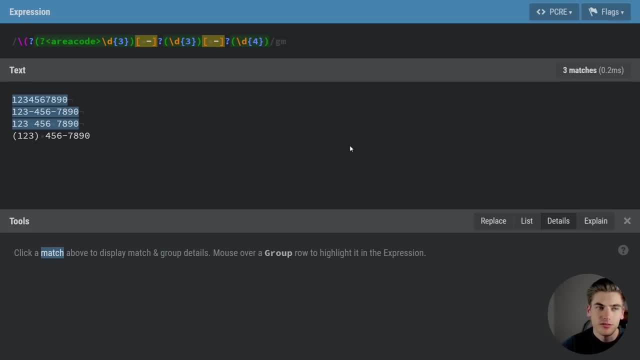 make sure that we do the backslash before, because this is a special character. So we have optionally one parentheses opening at the beginning, And then here we're going to have optionally one parentheses opening at the beginning, And then here we're going to have. 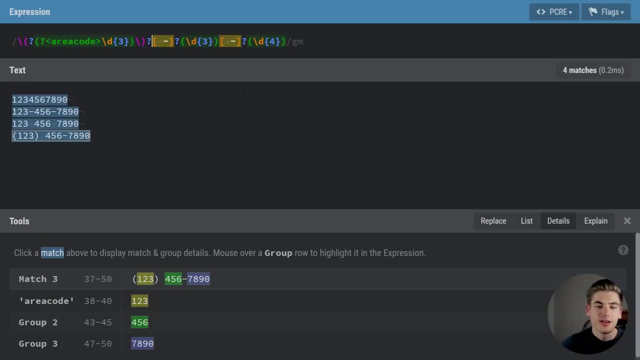 optionally one closing parentheses, just like this. And now you can see that it's working. And if we look down here our area code, 1, 2,, 3, we got 4,, 5,, 6, and then 7,, 8,, 9, 0.. Now one other. 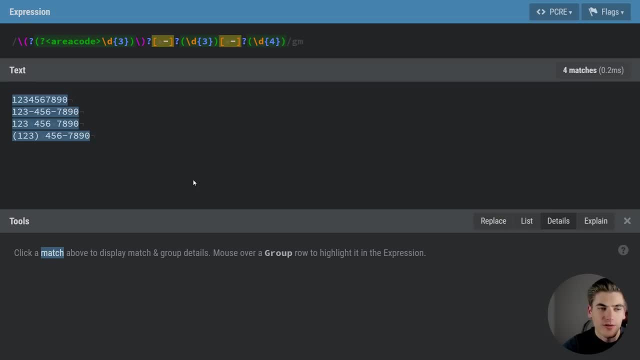 thing to account for is if you have international numbers, you're going to have, for example, a plus 1 at the beginning of the number, So we can have plus 1, 1,, 2,, 3,, 4,, 5,, 6,, 7,, 8,, 9, 0.